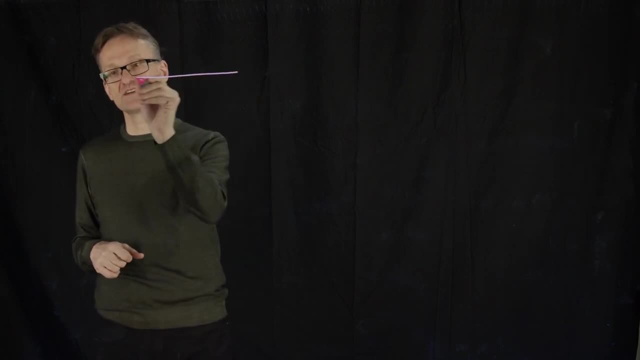 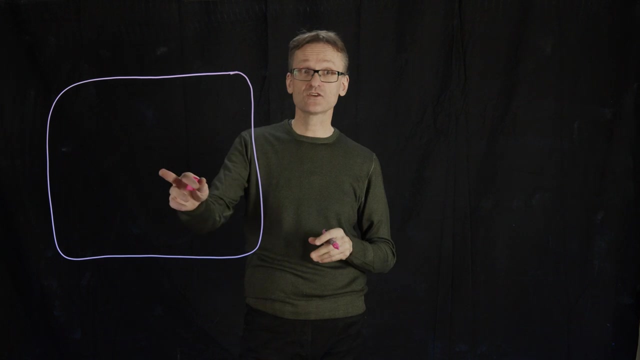 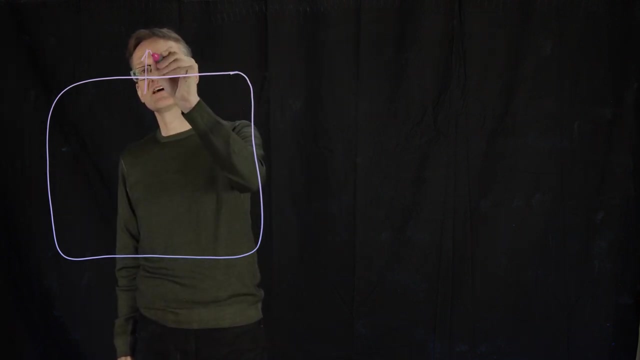 physicist, I love to study isolated systems. I already mentioned that. So here's a system, and by isolated I mean that it's not really. it's not exchanging anything with the outside, It's not exchanging particles and I'm not changing the shape of it or anything. So the only thing that 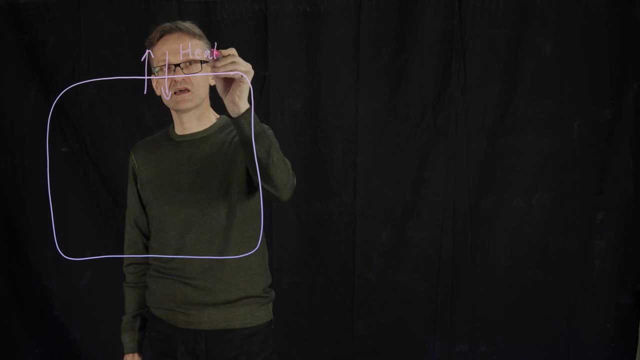 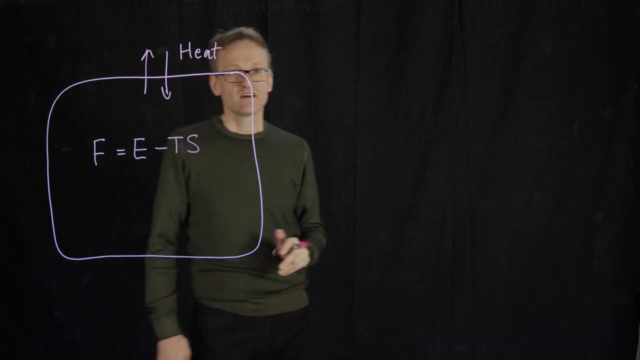 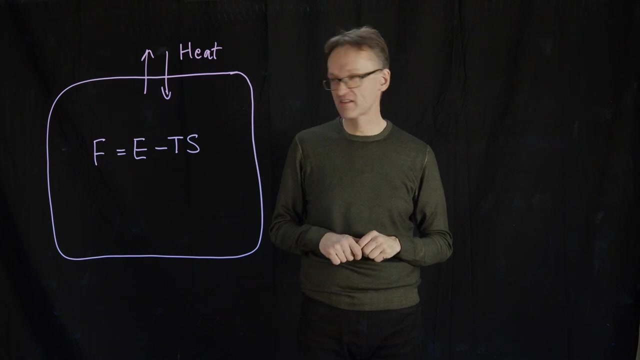 will go out or in of this system is heat Energy. in terms of heat, That means in the system I have my free energy. F equals E minus T s. Now, if that was the real world, things would be simple. The only problem: in the real world: things aren't that simple. 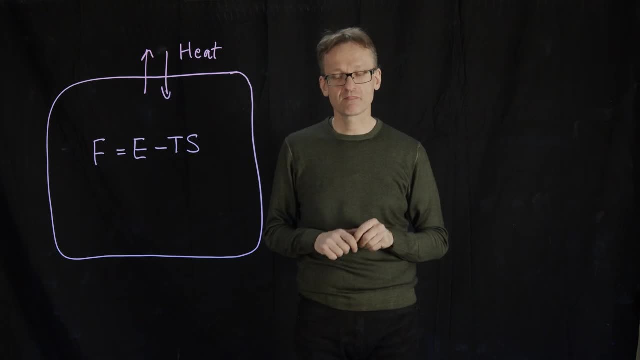 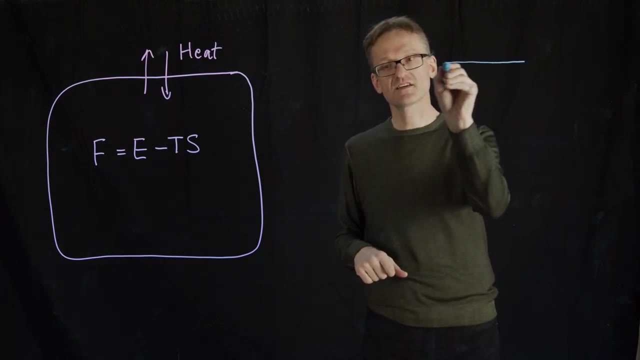 Rather. it is that simple, but there are very few systems we could study that way, So let's take my chemistry hat instead. Now I'm a chemist and a lab rat here. Here is the chemist system and I call this system. but imagine me sitting here and hauling a beaker or test tube. 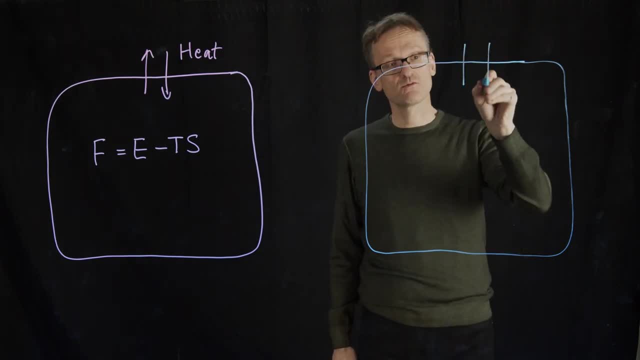 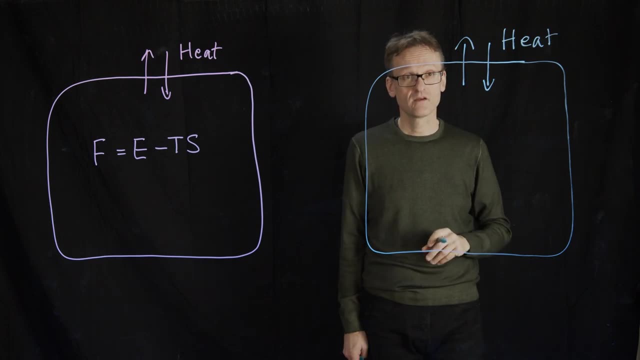 Sure, I too am exchanging energy with the rest of the world, and heat. That happens all the time. if I put this on a balsam burner or if there is a reaction happening that's heating the room. But what if I'm solvating a salt or something? The volume might actually change, because I have 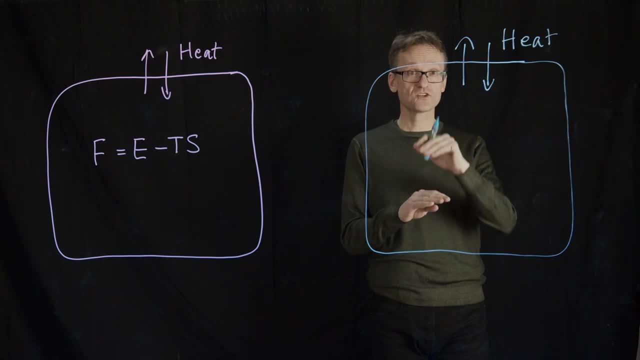 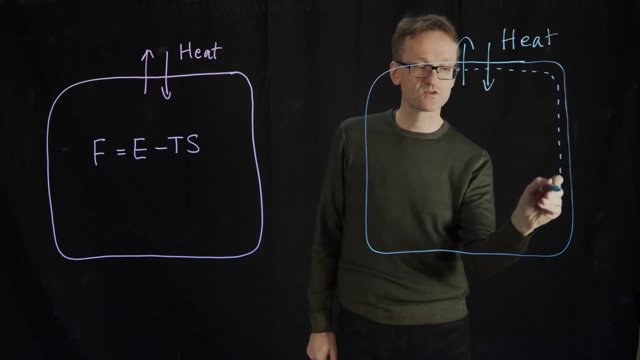 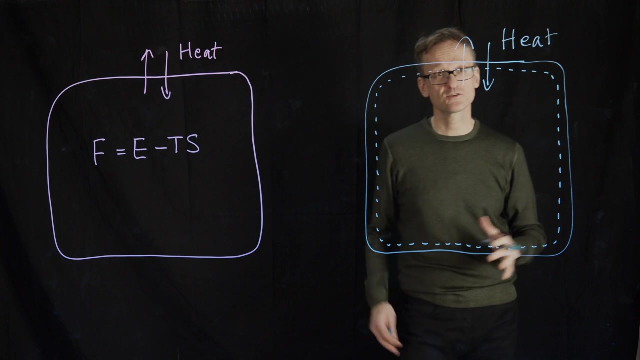 a test tube right, It's open. So if the pressure is changes, it can adjust the volume up and down. So here I'm going to need to account for the fact that my system might become smaller or larger because I'm performing. either I'm performing work on the outside world if I'm expanding, or 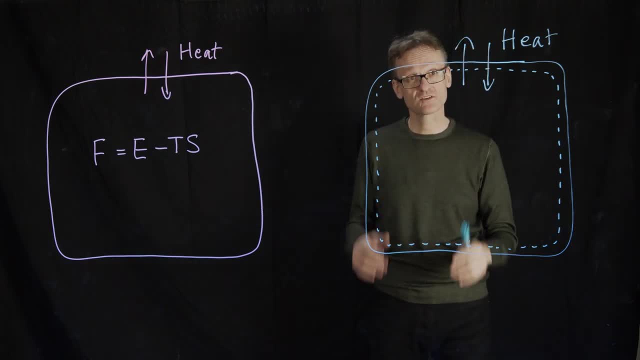 I let the outside world perform work on me. if I'm contracting the system To the physicist, this is a royal pain in the a To a chemist. that's come on, you don't have a real world unless you can describe this. So we know exactly how much work it takes to change. 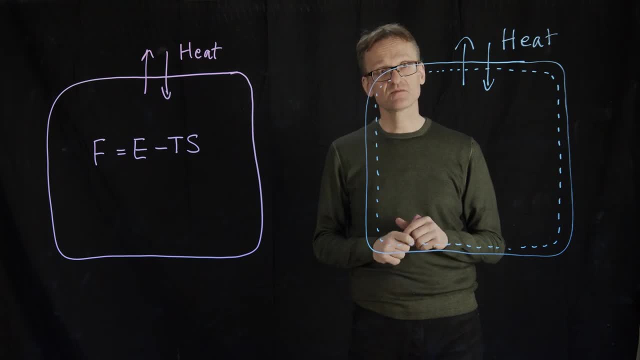 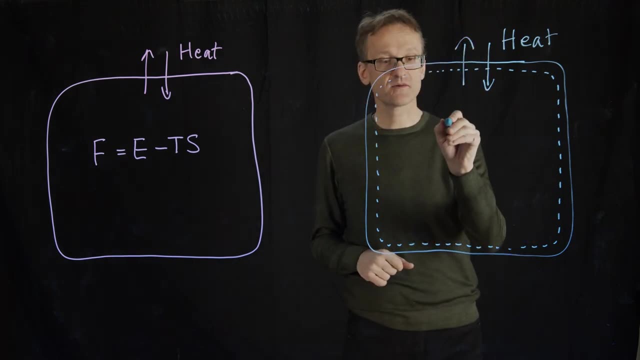 how much work it takes to change the volume of the system. v, That's the pressure multiplied by the volume. So the chemist is quite happy. We have a way to describe this. Leave some space here. So here I'm going to say that this is the work I do here is e plus p, v. 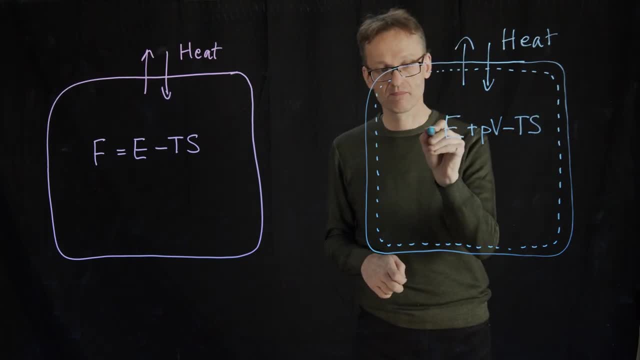 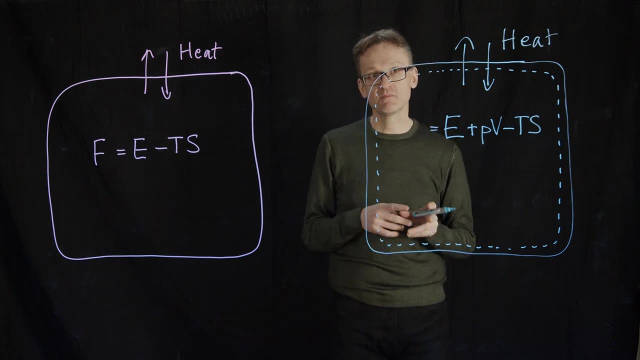 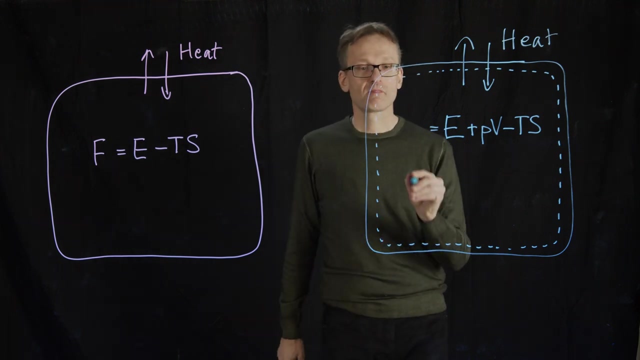 Minus t s. If we were astronomically stupid, I would call this f, because then I would have an f, but my f is not the same as that f And then you would always have to check: is the author and the chemist or a physicist? Let's call this g And this factor its energy and volume occasionally. 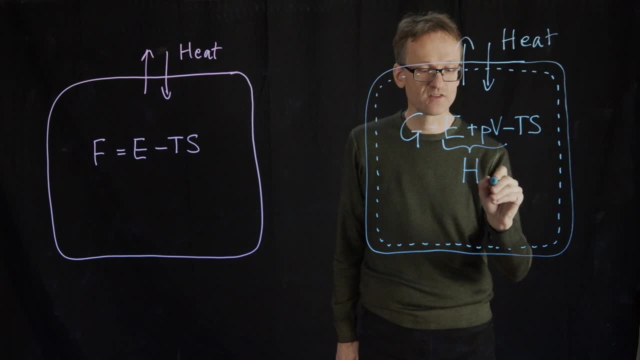 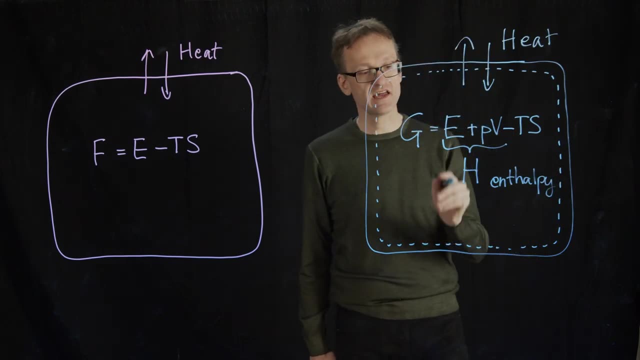 we call that h And the word for that would be enthalpy. So note: s is entropy, h is enthalpy. So enthalpy describes the internal energy of the system, multiplies the pressure, multiplied by the system's current volume, and that 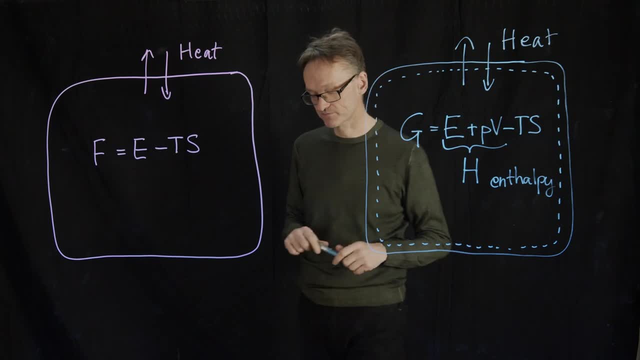 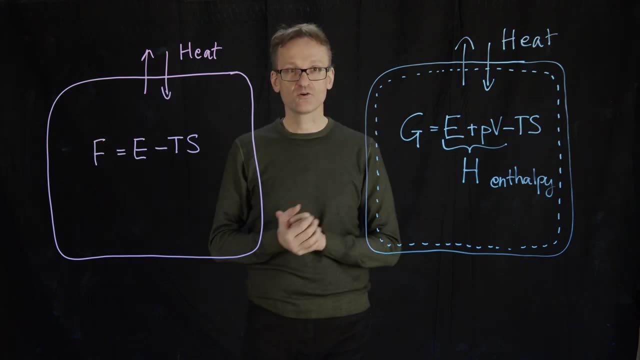 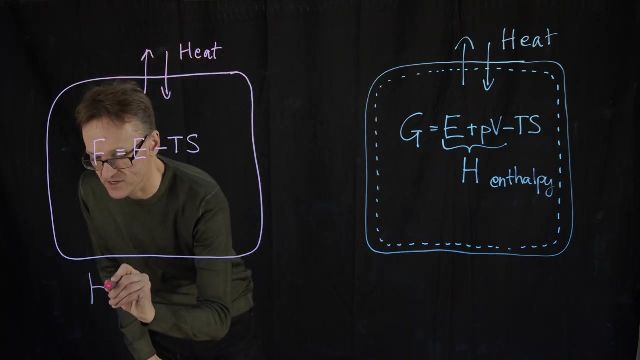 including that will account for the fact what happens if I change the volume of my system. Now, if the world was good, we would all be very careful and say: are we using f or a or g? The actually have names too. The physicist would say that this is the Helmholtz free energy and the 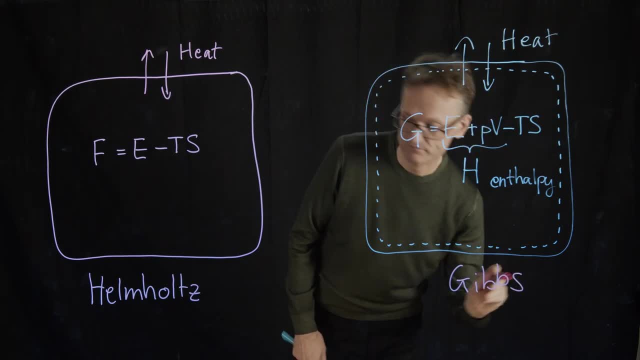 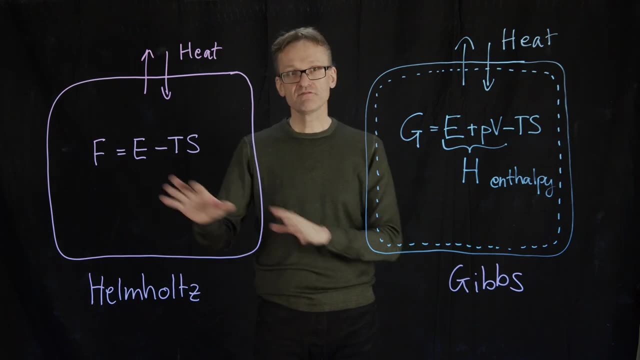 chemists would rather say that they're working with the Gibbs free energy. Occasionally we use A as a letter for the Helmholtz free energy too. F and A there on that side, G on that side. It's simple and beautiful world, right. Well, if it wasn't for the fact that occasionally, chemists 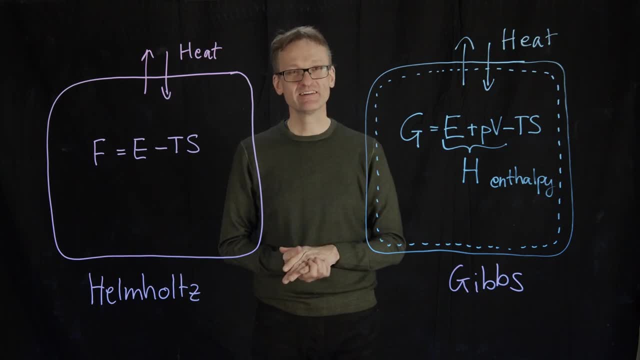 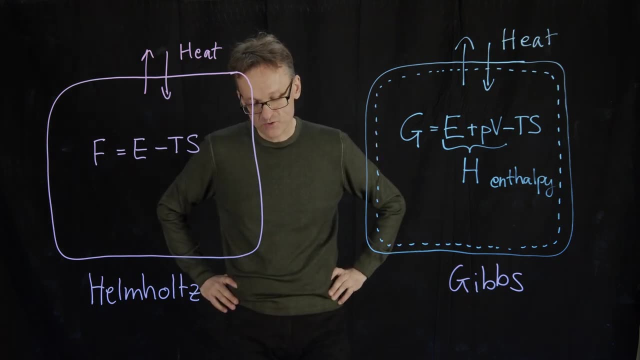 are sloppy and we use F for this one too, Sorry. Why on earth are we that stupid? Well, it turns out that for most reactions- let's say that I'm having one protein molecule fold- The volume change of that system is going to be one part in Avogadro's number. It's completely negligible. 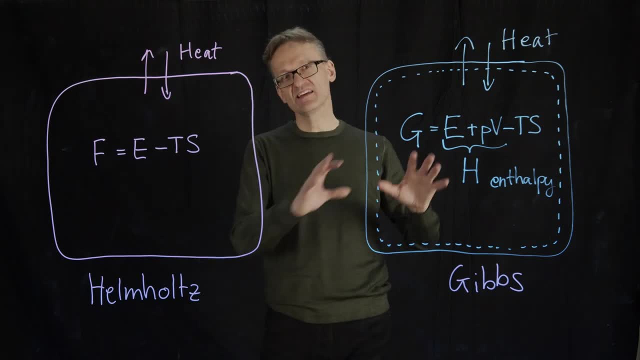 So that's short. Technically, formally, it is correct that I have to include the PV term here and everything In practice. I very rarely calculate the absolute values of things And if I'm only calculating a delta, a change, the delta in the PV term is going to be so small. 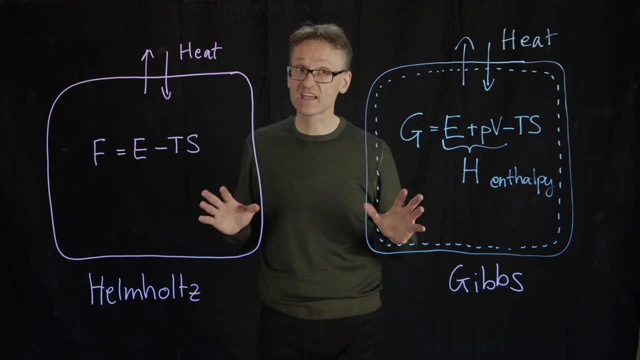 that I can always say that it's zero Again, not for any chemical reaction, but for reactions if I'm solvating a protein or breaking a hydrogen bond or something, And that means that you will occasionally see even me right: F equals H minus TS, or F equals E minus TS. Sorry, just deal with it. You need to understand the